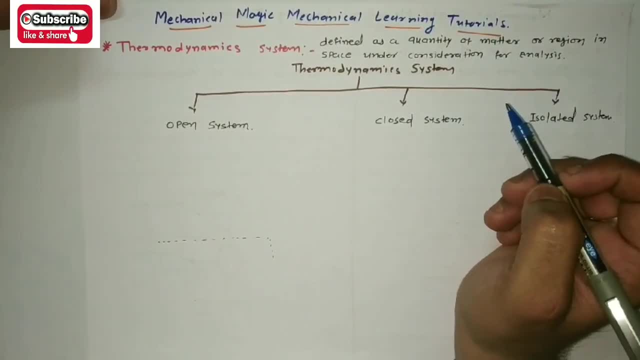 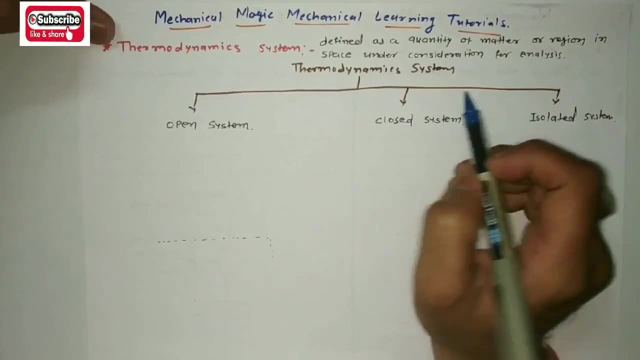 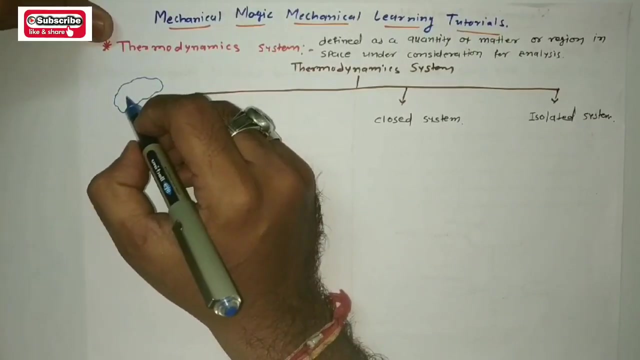 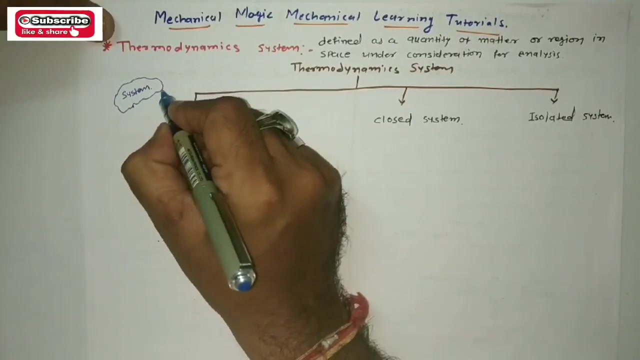 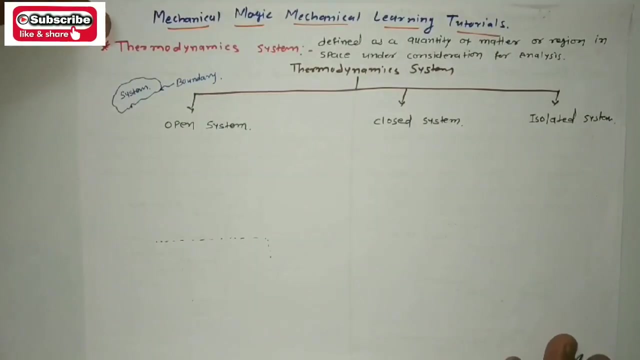 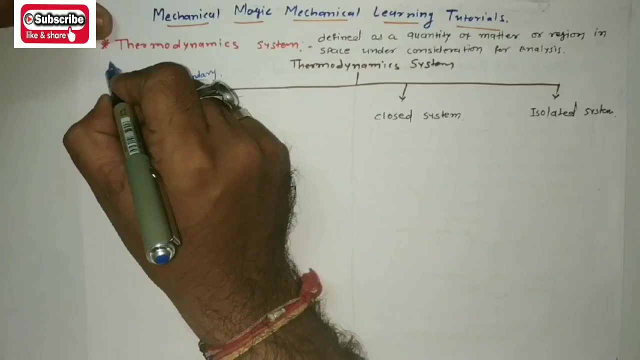 So basically thermodynamic system, that will be into category of the three systems. So in that case, thermodynamics, basically there is a one system and that will be having a boundary, So boundary is separated, that system from the surrounding, So outside that will be surroundings. 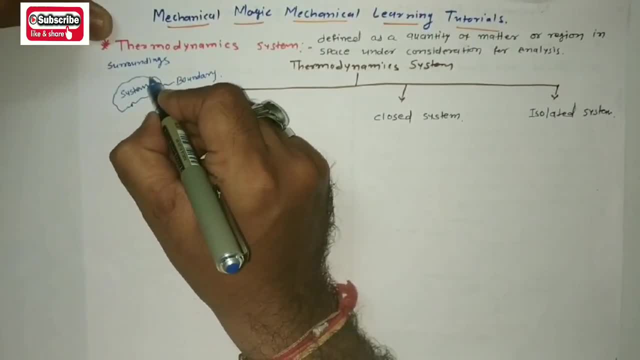 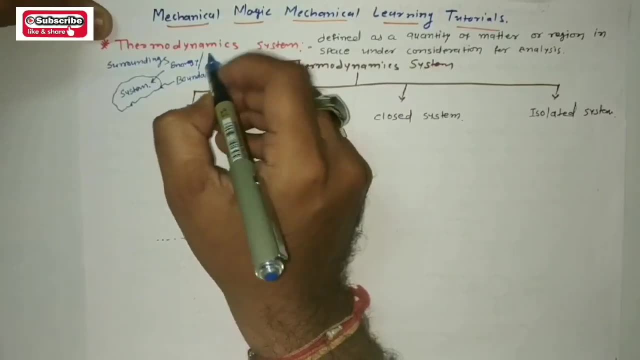 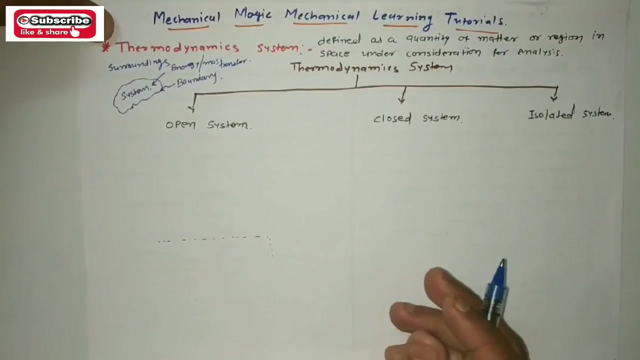 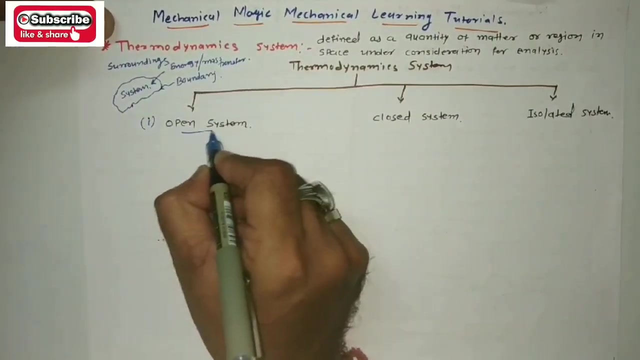 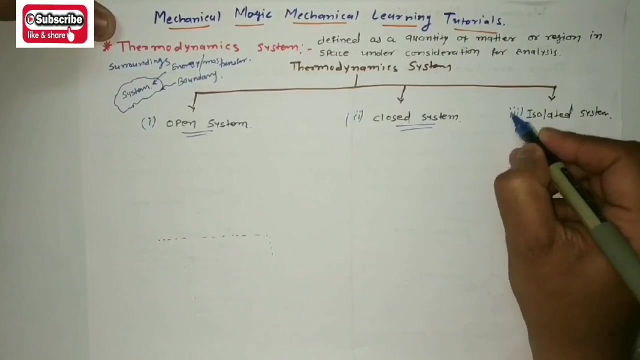 So you can say system to surroundings or surrounding the systems, there will be some amount of energy, or you can say mass transfer. So in the case of thermodynamic systems, basically that will be having a three category: open system, closed system and third, and that will be considering as a isolated system. 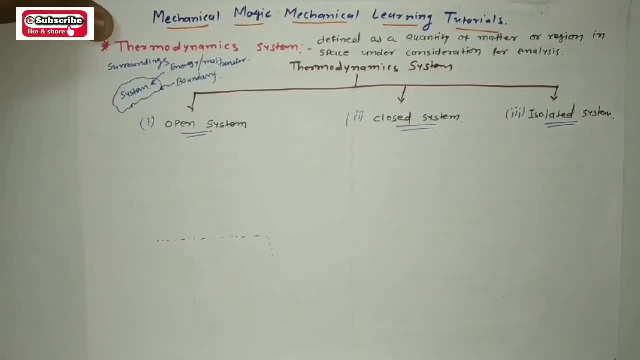 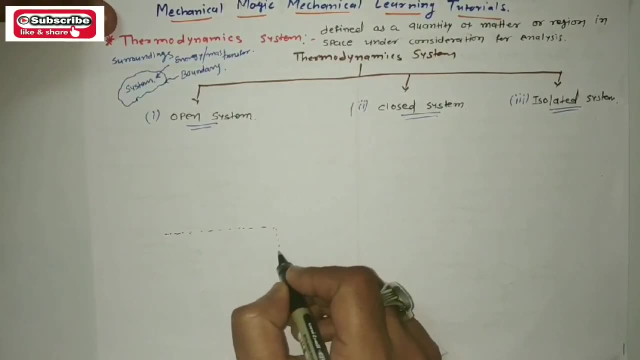 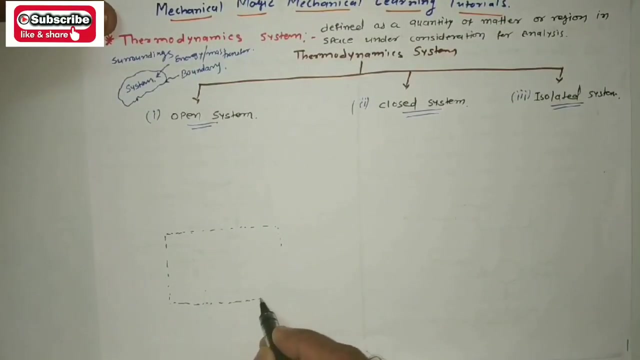 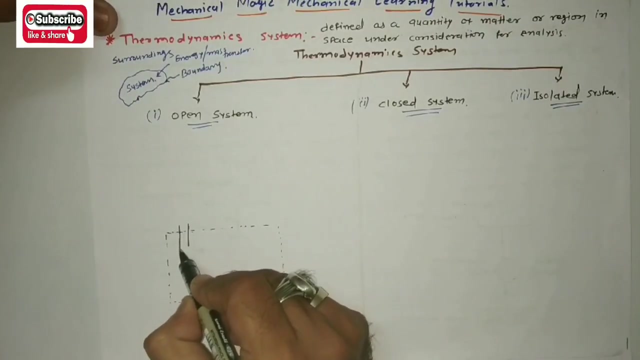 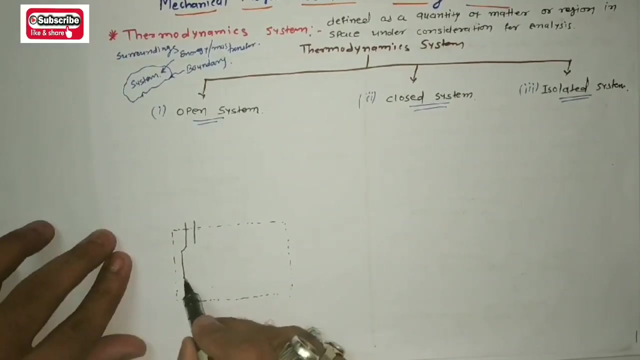 So let us see first open system. So in case of open system, One of the examples over here for turbine, and it will be like this, So just you can see This is a symbol of the turbine. So you can write down over here: turbine. 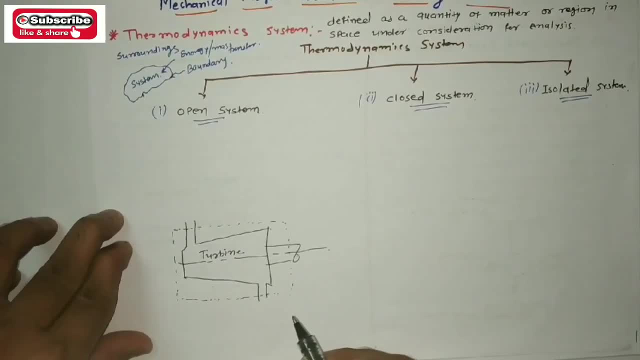 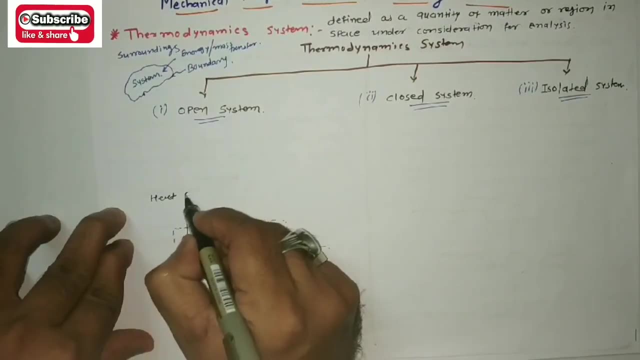 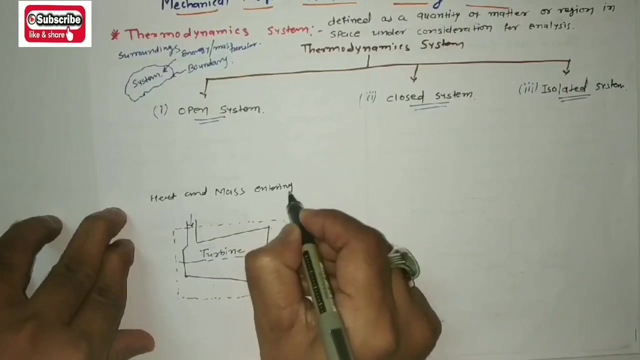 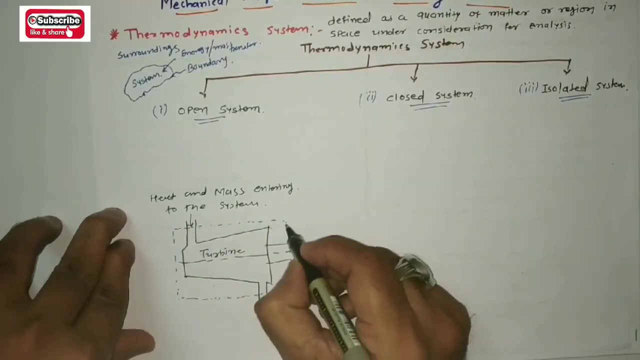 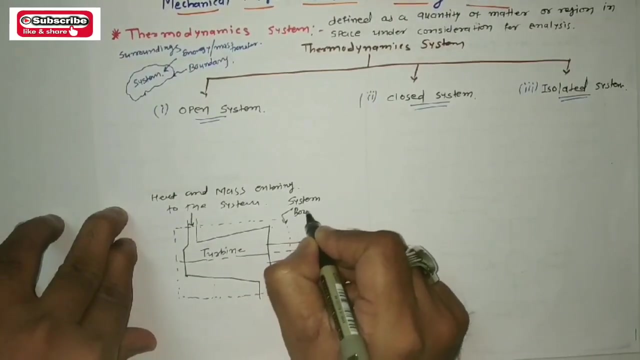 So in the case of open systems, from here that will be heat and mass, So it will be the material entering into the system. So then now, if this system is made of material justement, another else will be closed system. it will be representing the flow of energy from the system fast to the body. 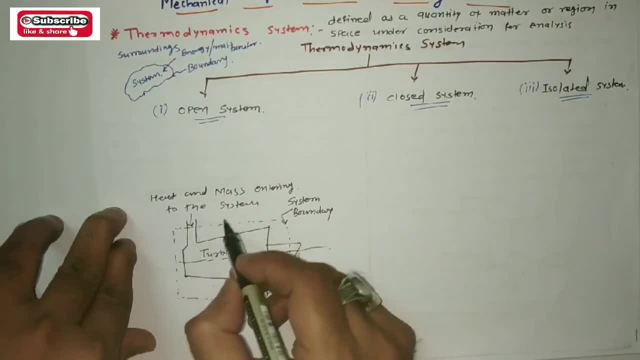 So all these four are are serving the mass of the energy that Preferably in this Eight types both of the heat sources of energy flow and then the system is heading itself And the reactor is represented as a system boundary And that will be representing is 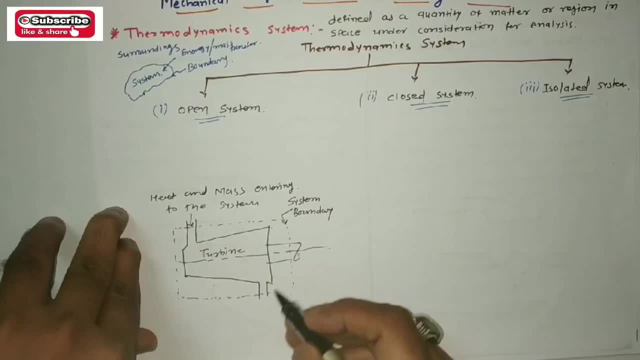 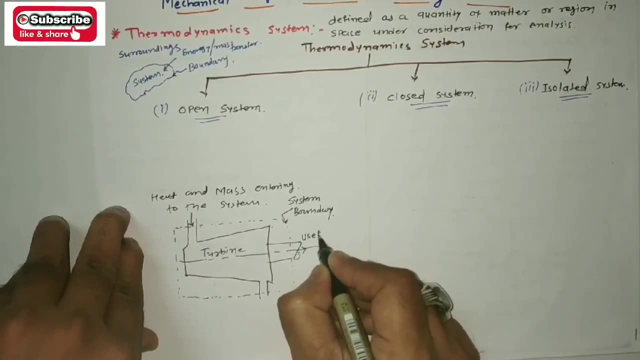 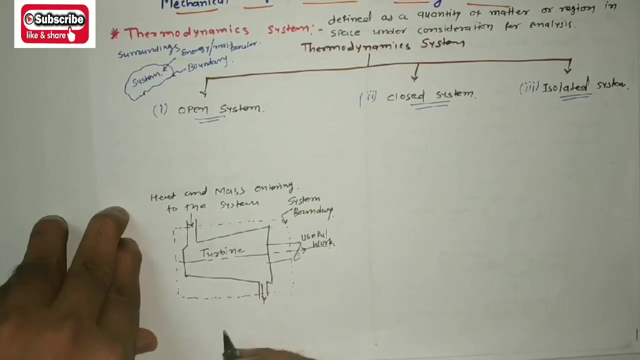 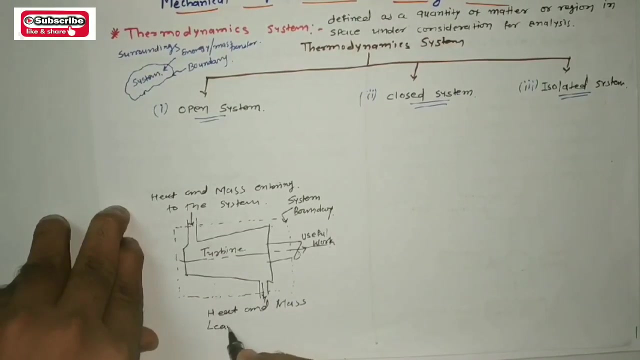 say that energy it will be converting into the rotation and that will be coming out from that particular shaft. So you can say that use full work and rest of the heat and mass that will be reliving from the another end. So you can write down over here heat and mass. 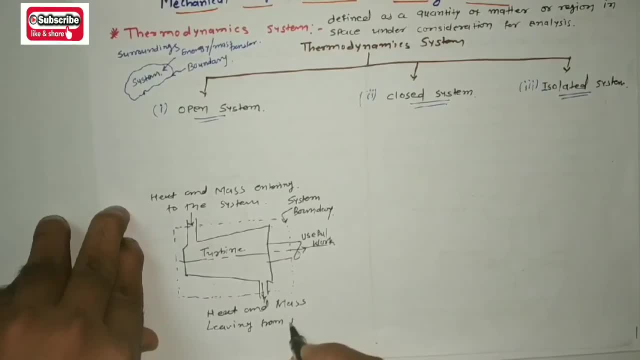 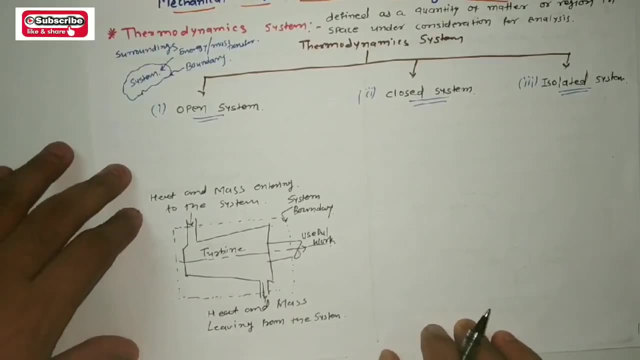 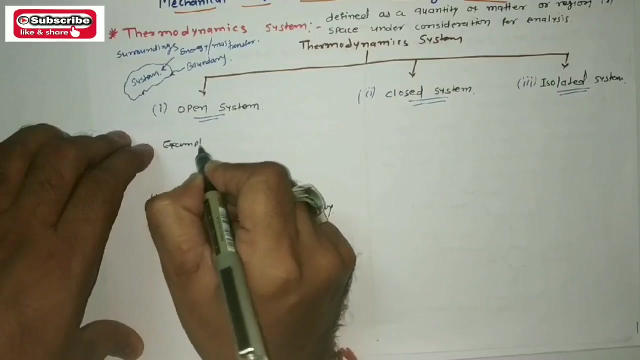 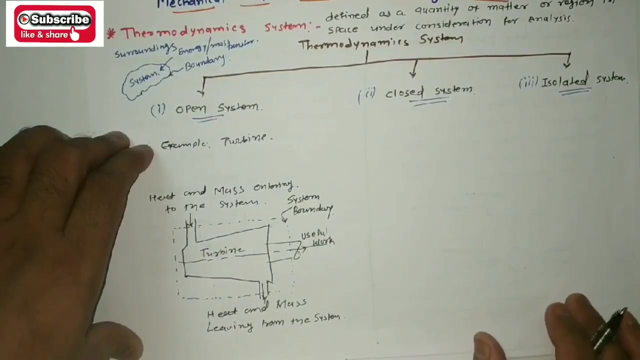 leaving from the system. So such kind of examples of the turbine that will be considering as a open system. or you can say example of turbine, So now you can also considering as a IC engine as a example, an open systems. But now I want to talking about a closed systems. So in that case which? 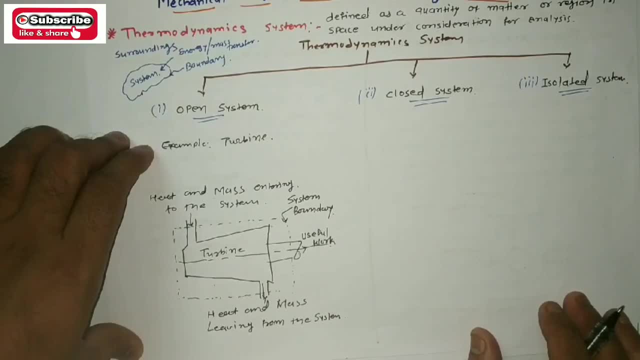 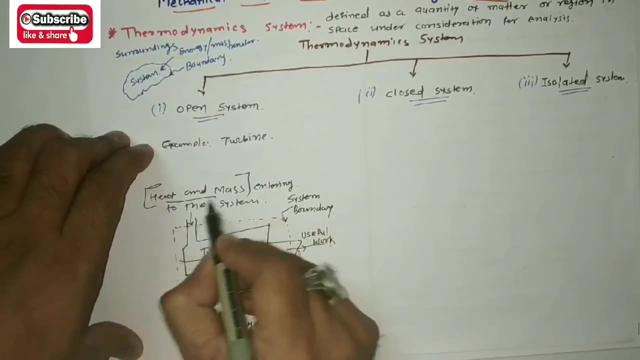 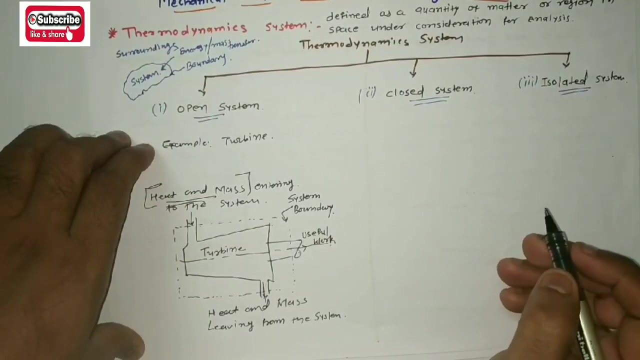 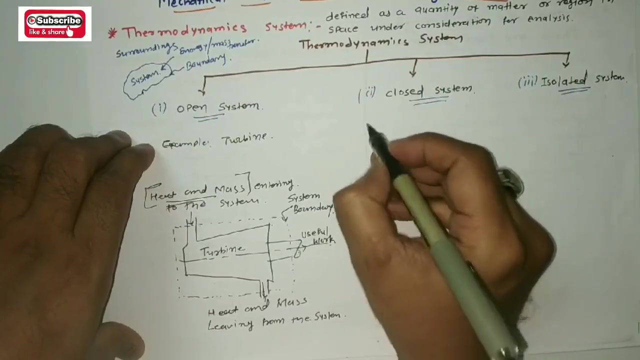 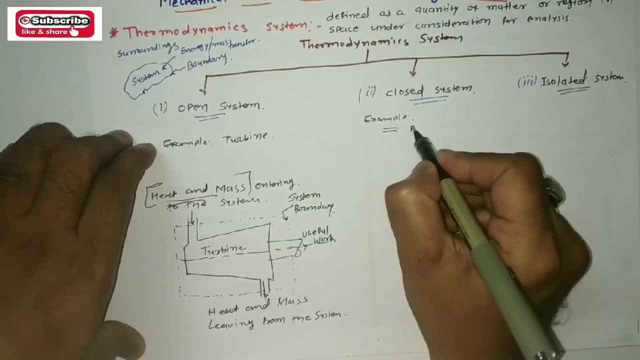 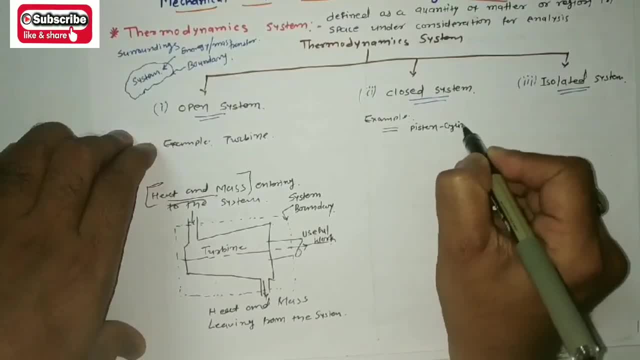 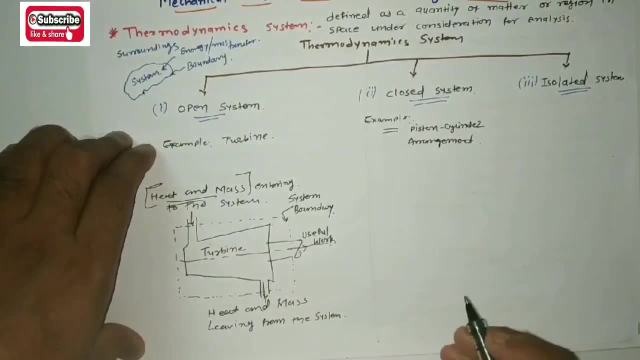 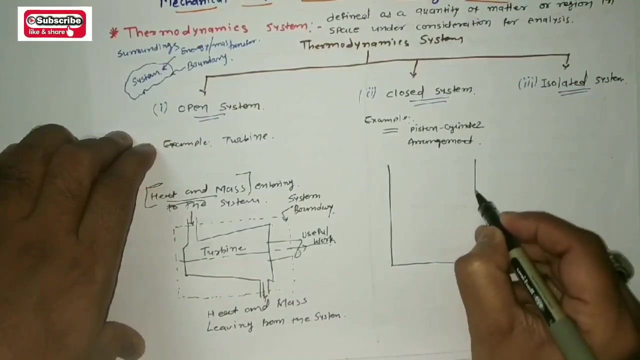 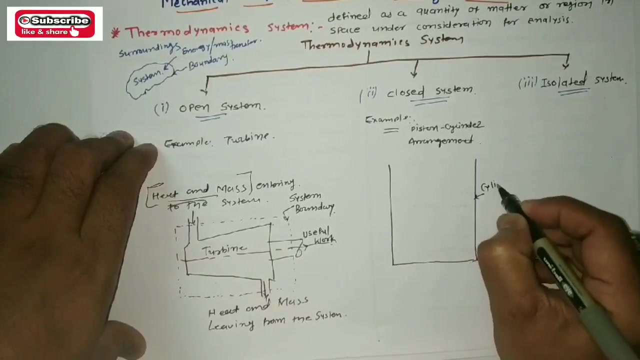 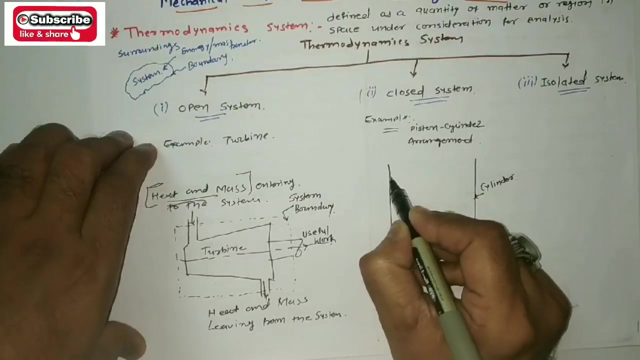 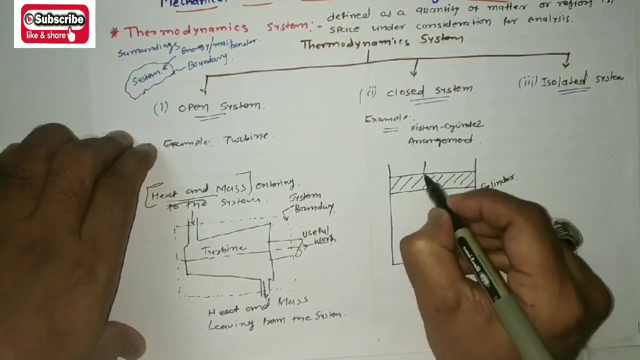 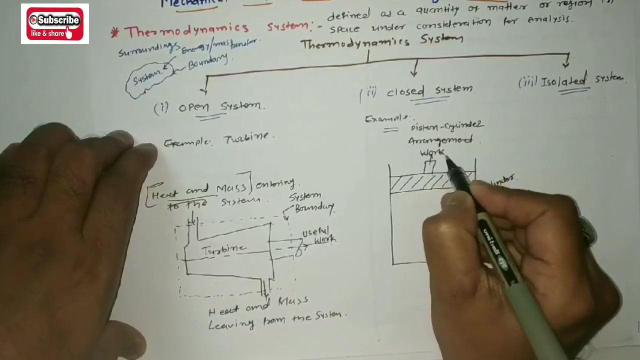 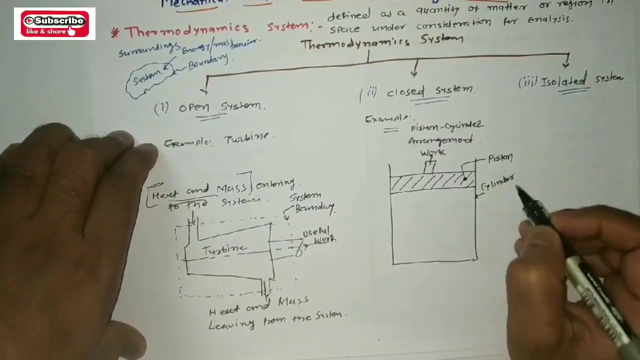 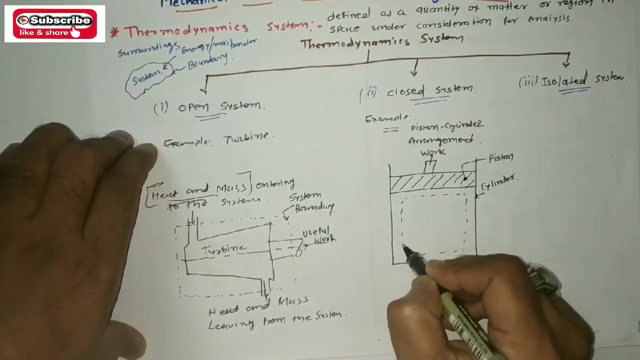 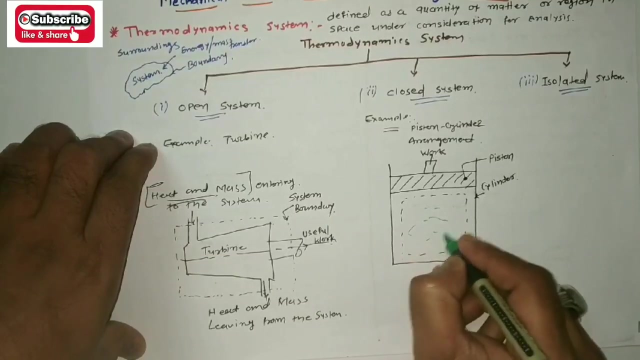 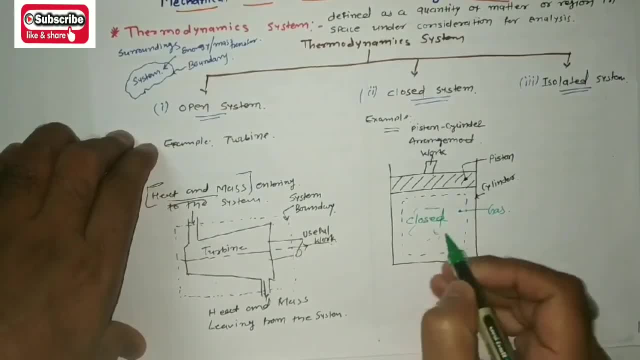 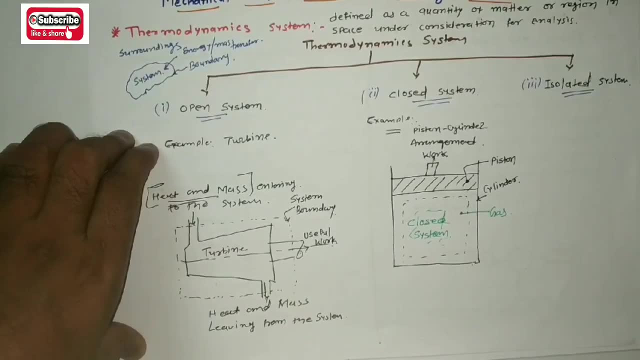 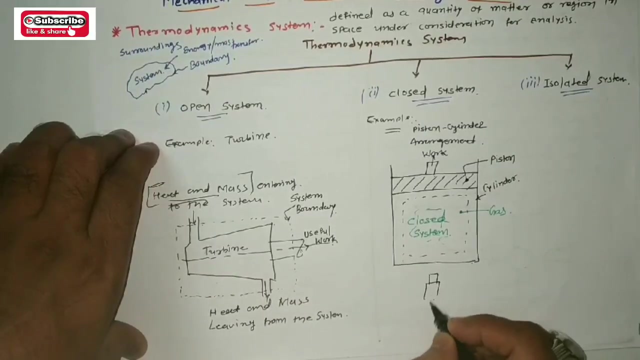 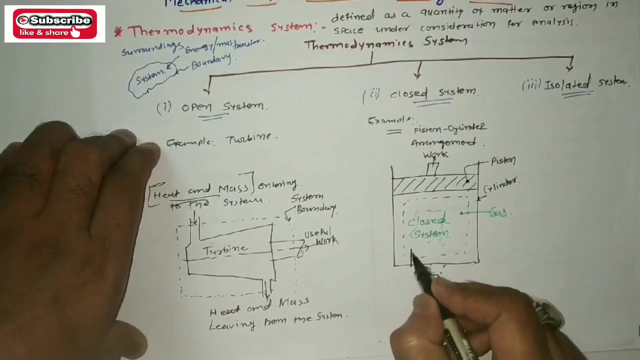 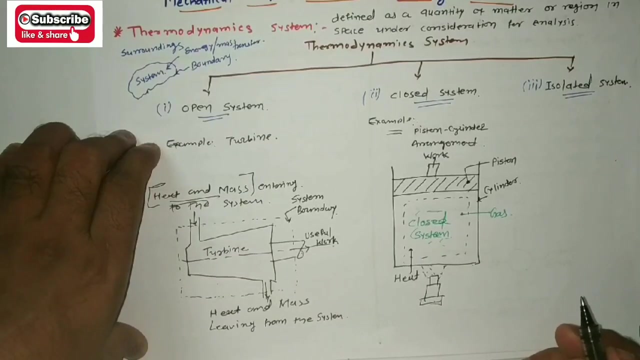 say it will be the closed system, so with the help of burner kind of arrangement, that will be heated. or you can say heat is supplied, So generally energy is transfer. or you can say heat in the form of energy, So only heat is supplied to the systems and rest of the part here that will be. 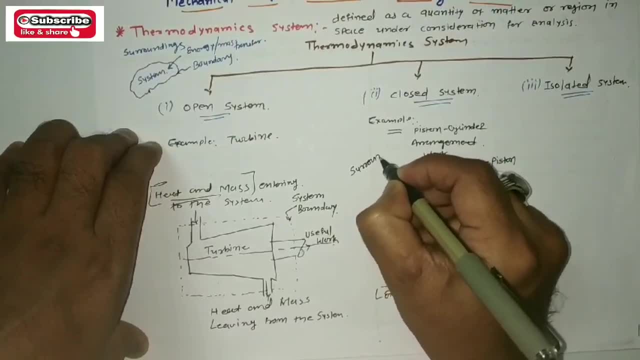 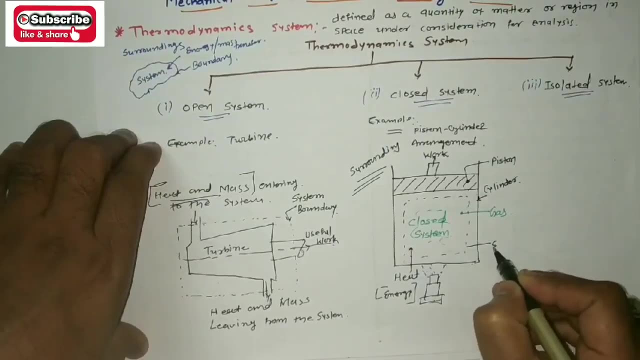 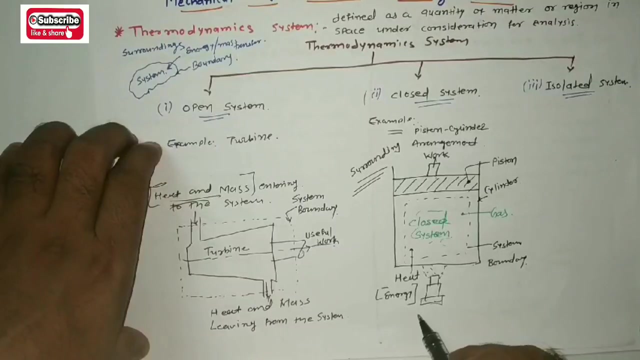 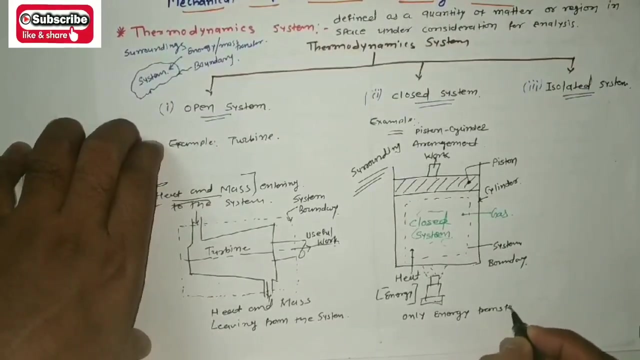 considering as a surroundings and that would be considering as a system boundary. So here, by the increasing of a temperature, you can say, or in the form of heat energy, so that will be increasing the pressure of the gas, but there is no any kind of mass transfer during the process. So in that case only energy transfer at its 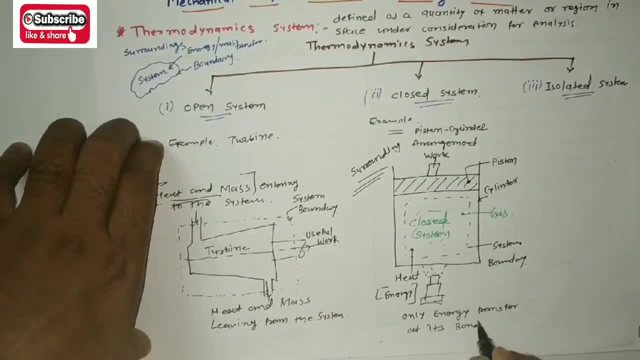 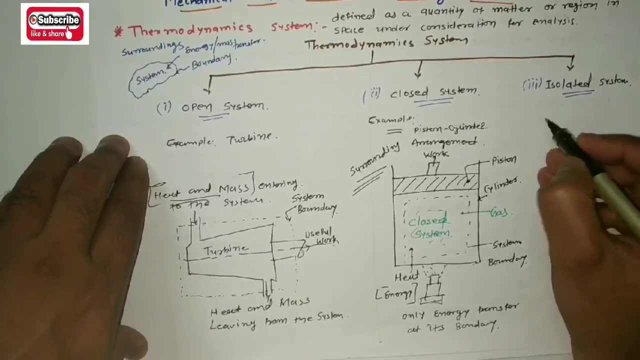 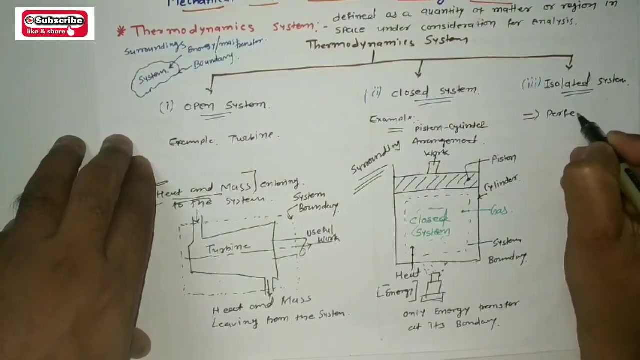 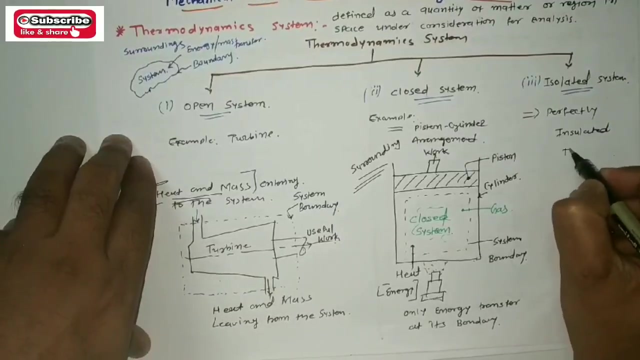 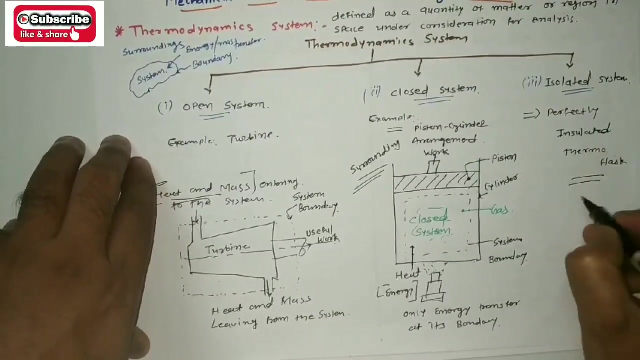 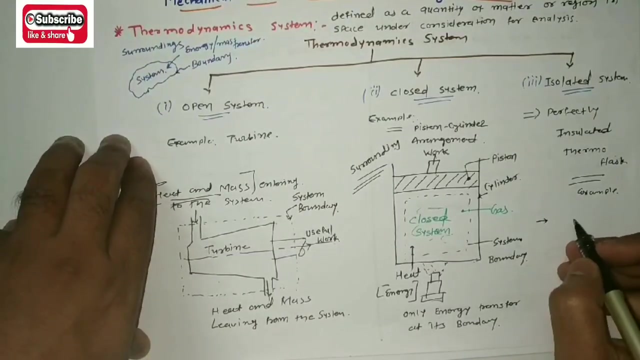 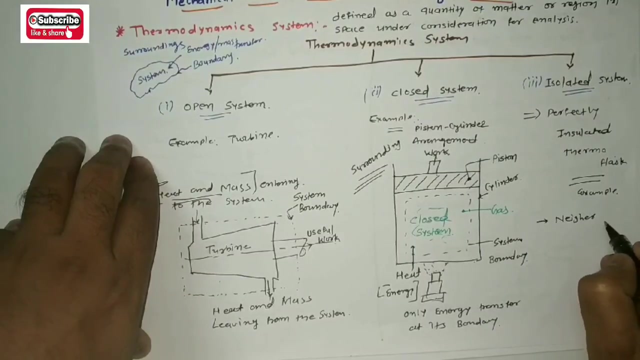 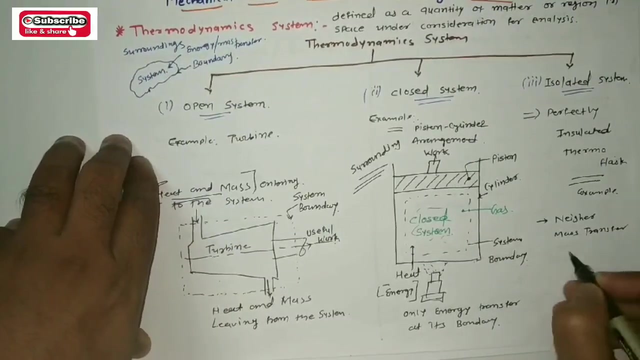 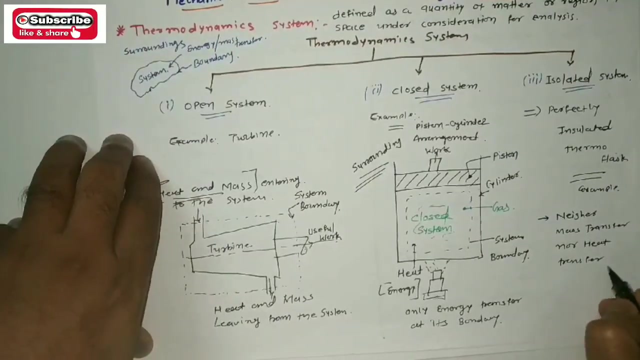 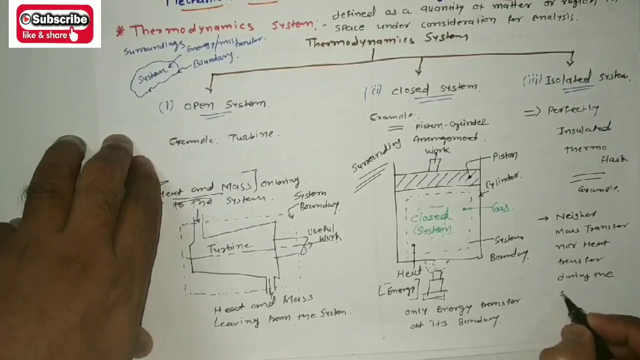 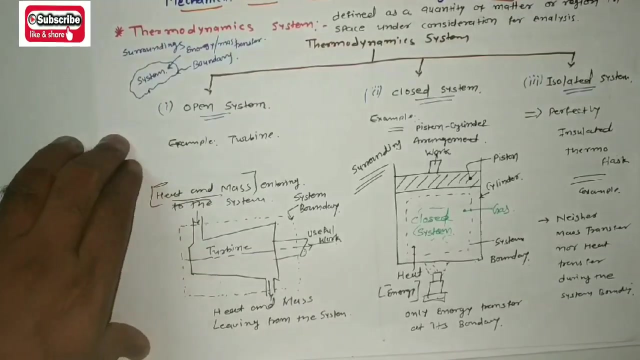 boundary. So last one: isolated systems. or you can say perfectly insulated thermo flask, So that will be the example of isolated system. So in technical language you can say that neither mass transfer nor heat transfer during the motorization process, or you can say at the system boundary, so that will be considering as a isolated system. so in